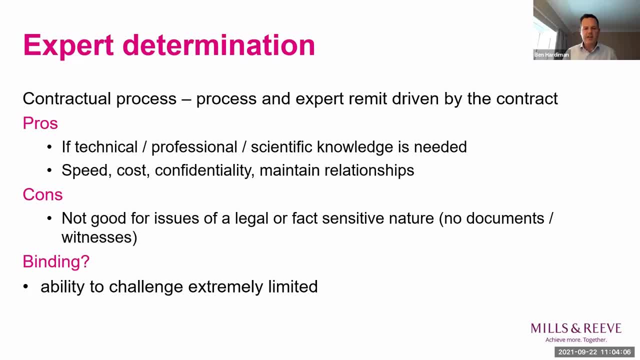 expert determination? Yeah, I think there are. The problem is that, as I said earlier, this is a contractual mechanism. so the scope of the procedure, potentially even the identity of the expert to be appointed and that person's remit, are all driven entirely by the provisions of the contract. 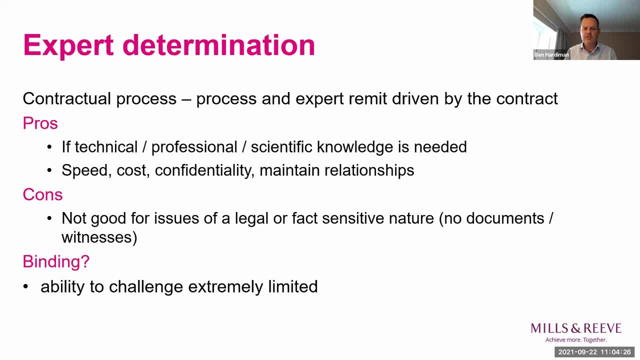 So the main downside is that when the parties enter into the contract, they don't necessarily know the scope of the potential dispute, which may not arise for several years, And that can mean that an expert determination process is entirely unsuited to the dispute that later arises. but by the nature of the contract they're bound into it. Secondly, and as I put on, 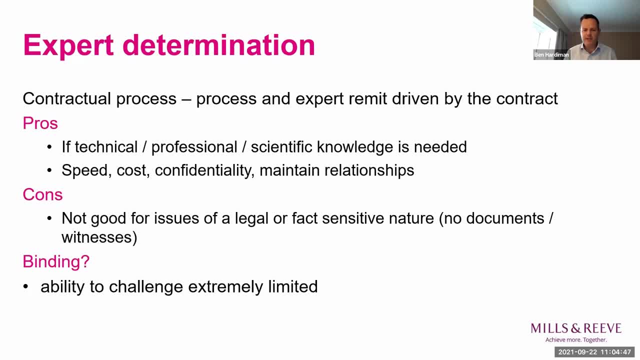 the screen. this is perhaps a bigger issue from a construction perspective, which is it is less suited for resolving claims which involve factual disputes and which are going to involve some review of documentary or witness evidence. It's also not good where there are particularly complicated legal issues involved, because more often than not, by their very nature, an expert is. 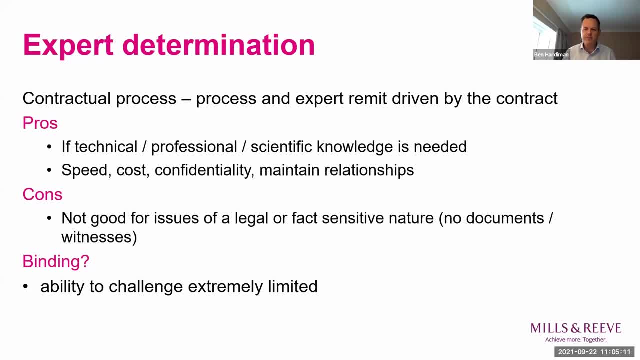 an expert and not legally qualified, so may well not be able to provide the input into those parts of the dispute. Thanks, Ben. And what would you say are the main benefits of using expert determination? Yeah, there undoubtedly are some. I shouldn't cast dispersions completely. 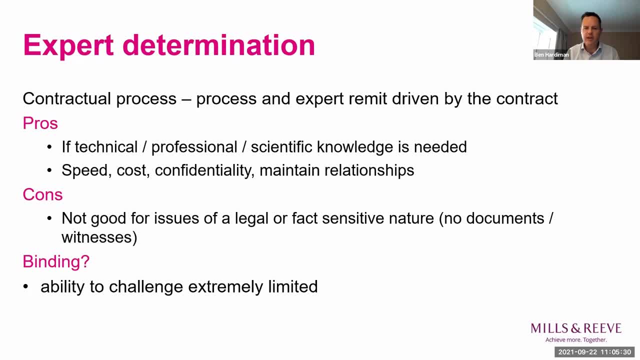 It's less formal than litigation or arbitration, so it's generally quicker. it's generally more cost effective. It's also a confidential process, so it offers the parties a way out of a dispute whilst giving the chance of preserving an existing relationship. Also, the benefit it gives is having 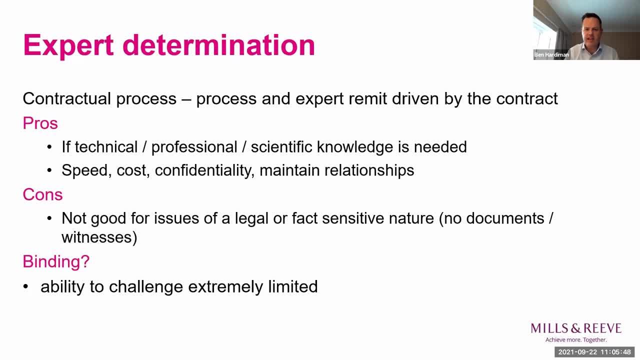 an independent party with specialist technical knowledge and perhaps familiarity with the problem that's arisen, that can give a decision which enables the parties to walk away knowing that the outcome can at least be objectively justified because someone who knows the issue is has made a decision. So just talking about a decision, a key question is: is expert determination? 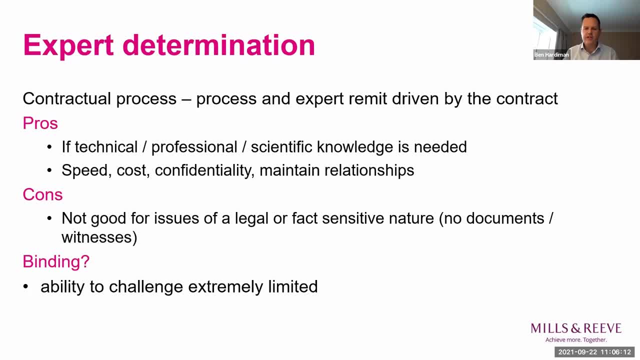 binding? A classic lawyer's answer for you on this one, Andrea. The answer is not completely straightforward. I think the answer is ultimately yes. The reason for a caveat is there's very little established case law relating to expert determination, because it's far less used. 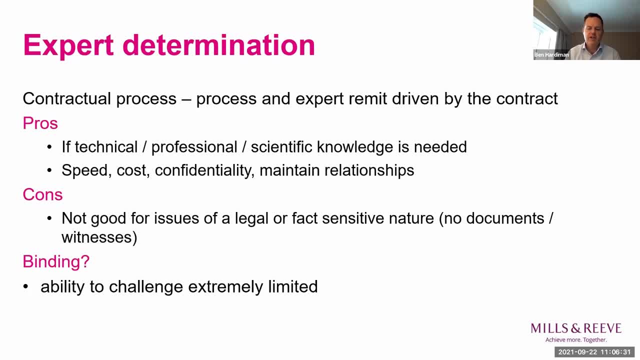 than the likes of arbitration and adjudication. I think the answer is that there's very little, but where issues have come before the courts, generally judges have taken the view that an expert's decision is binding and shouldn't be interfered with because someone with appropriate 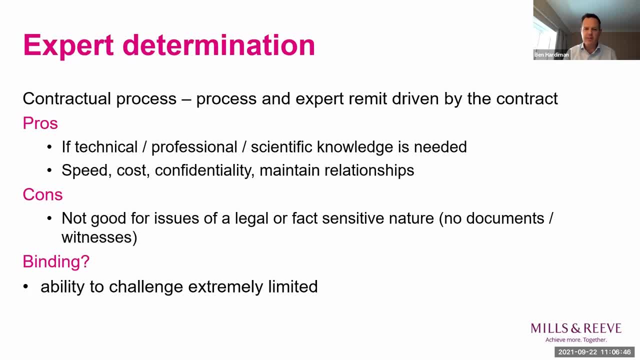 knowledge and expertise. who's been appointed by agreement of the parties, has reached a reasoned view. So, in reality, the ability to challenge is very limited. The right to appeal is virtually non-existent If you don't like the outcome. the reality is you're pretty much stuck with it. 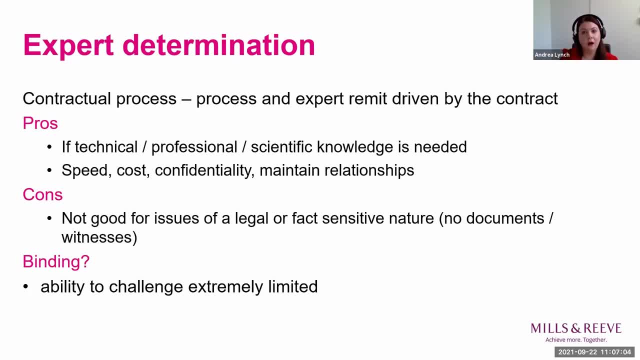 And finally, Ben, when you've got the determiner's decision, how then do you enforce it? It can't be enforced without court action. so the mechanism is: the decision becomes part of the contract. so if there is a failure to comply with that decision, that amounts to a breach of 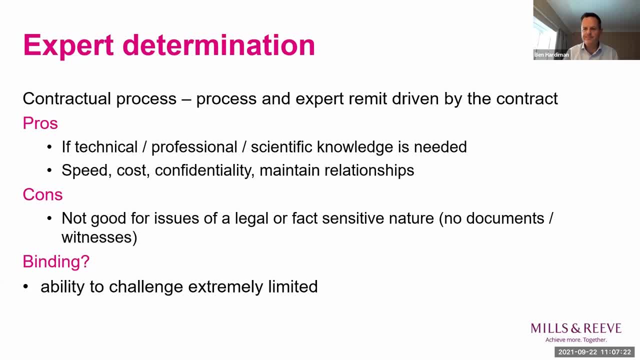 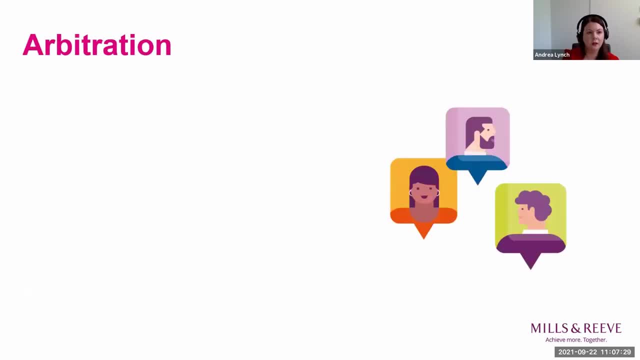 contract, that means you have to go through the courts to enforce it. Great thanks, Ben Turning. now to the, the second method of dispute resolution we're going to talk about this morning, which is arbitration. Again, Again, this is one of the less common forms of dispute resolution that is utilised in a construction setting. 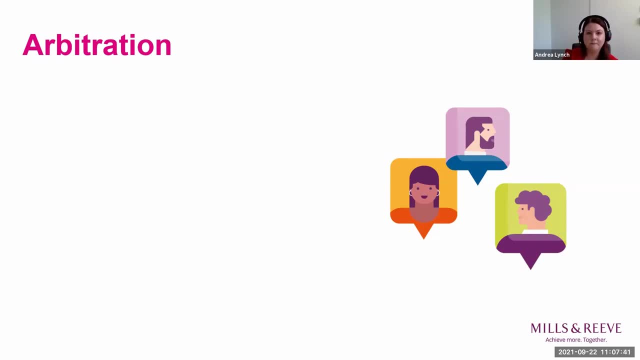 Andrew, can you explain to our attendees what exactly arbitration is? Thanks, Andrea, And good morning everyone. So yeah, arbitration is obviously an alternative to litigation and it's based on the party's agreement, So all parties to the dispute must agree to submit it to arbitration. 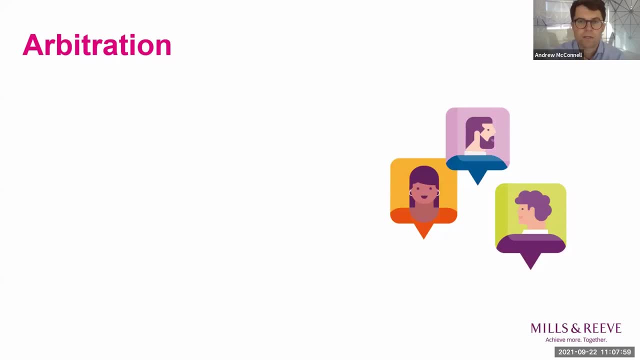 And like a judgment, the decision of the tribunal is a final and binding one. And what are the usual drivers for parties when choosing arbitration? So you'll see from the slide. I've sort of broken it down into four main objectives, if you will. 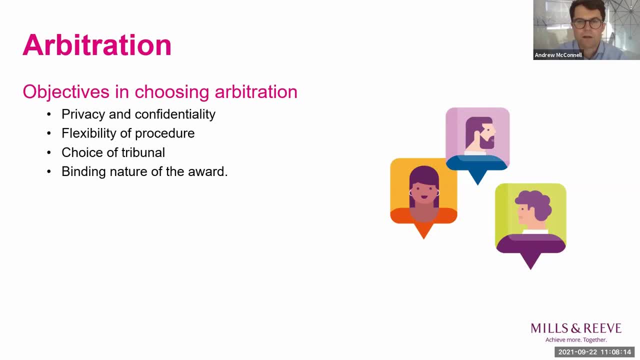 So the first one is privacy and confidentiality, So, unlike court proceedings, the parties to an arbitration abound by a duty to confidentiality. The second is the flexibility of procedure, So parties have the power to agree to a particular procedure that suits their needs for the case in question. 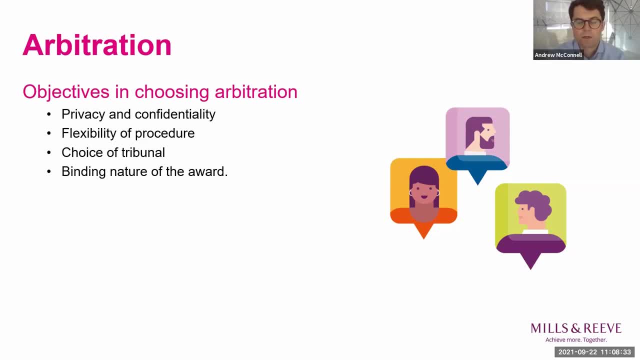 The next point is obviously the choice of tribunal, So the parties can choose a tribunal with relevant expertise, which is obviously quite important when we're looking at quite specialised and technical construction disputes that we advise on as a team. And, finally, the award is final and binding, as I alluded to earlier. 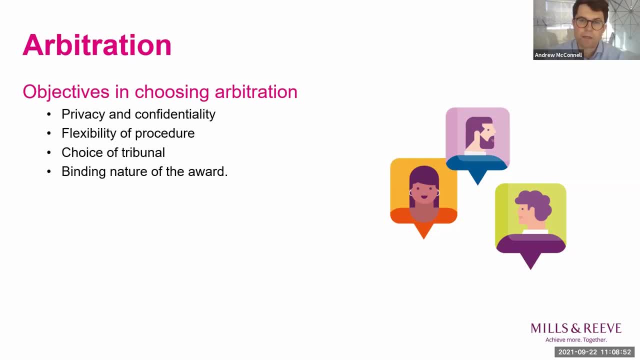 And there are very, very limited grounds on which to appeal the decision of the arbitration tribunal. Thanks, Andrea. Are there any procedural points that people should consider before commencing an adjudication? Yeah, there certainly are, And I think the parties always need to consider applicable time limits. 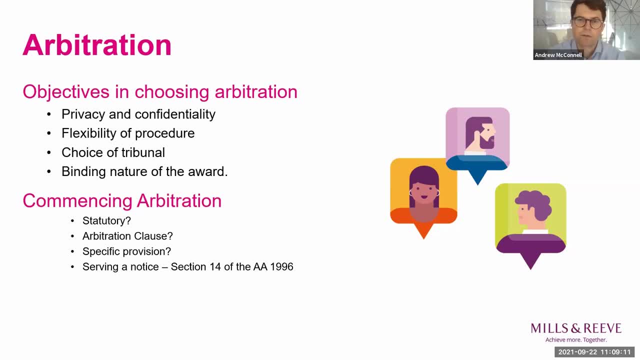 So the parties, or the same statutory time limits rather apply to arbitration proceedings as those for civil court proceedings. I won't go into those now, That's probably an entire seminar on its own, but the parties should be aware of limitation. 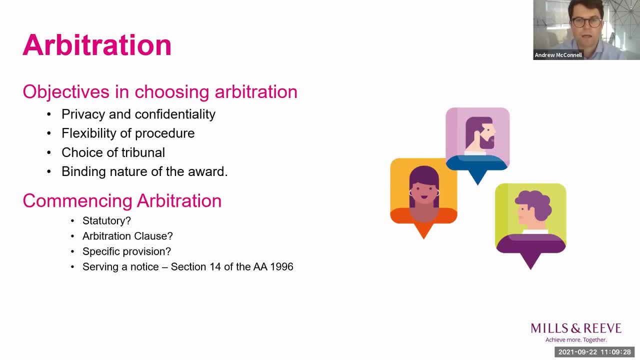 Alternatively, if there's an arbitration agreement, it might contain a clause that requires arbitration proceedings to be initiated by a certain time. The parties should also confirm the necessary steps in order to commence an arbitration, which may include things like making a claim, nominating a specific arbitrator or indeed just notifying the other side of your intention to arbitrate. 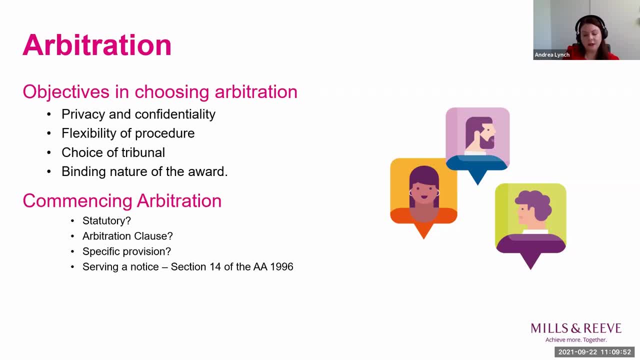 Thanks, Andrea. I mean out of interest. why do you think it's one of the less commonly utilised forms of dispute resolution in a construction setting? Well, probably several reasons, Andrea, but I think it's primarily because arbitration is final and binding, as I've mentioned several times now, which leaves very little room for negotiation between the parties. 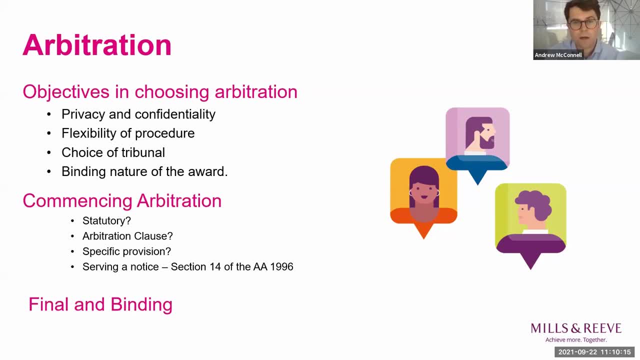 It can prove costly in terms of costs for lawyers and the arbitrator themselves, And there are other forms of ADR available which are potentially more cost effective and quicker forms of resolution, And we'll obviously come on to those later today. Great Thanks, Andrea. 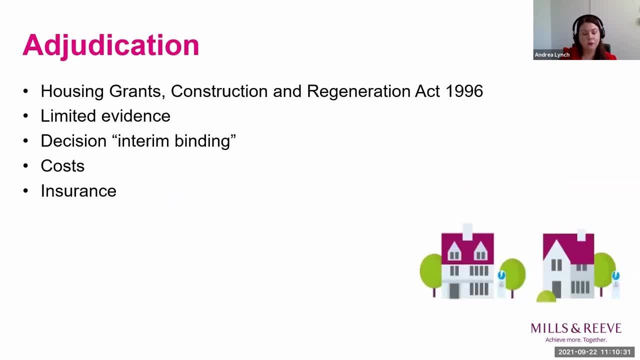 So, turning now to the next form of dispute resolution, which is adjudication. I know that a number of our attendees have expressed that they've experienced this previously, So the first. We're just going to run a quick poll before I turn over to Ben. 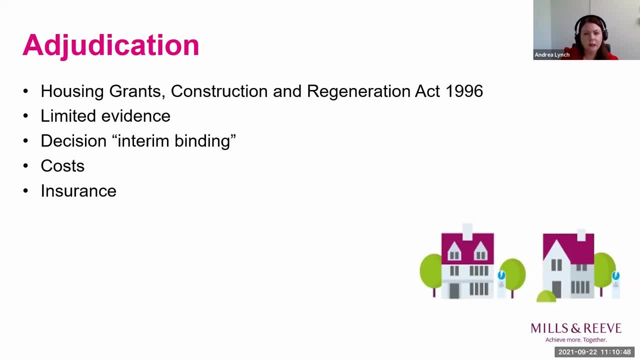 So typically, how long is an adjudication procedure? So we have four answers there. So one: no time limits. two: 28 days, three: 14 days or three months. It's quite a mixed bag. 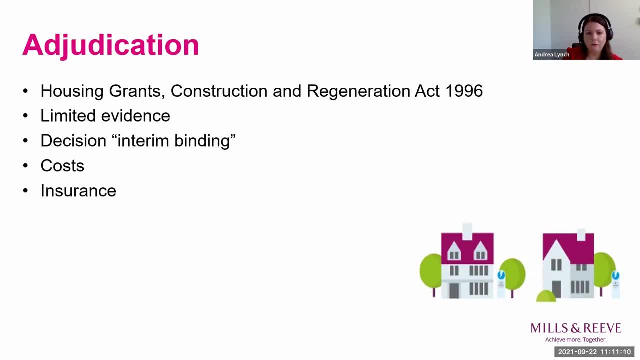 Most of you are going for 28 days but, Sorry, these are changing quite a bit. 11% think three months, 18% think no time limits. Ben, I think you'll come on to this to explain that, in principle, the idea for an adjudication procedure is that it will start and finish within 28 days. 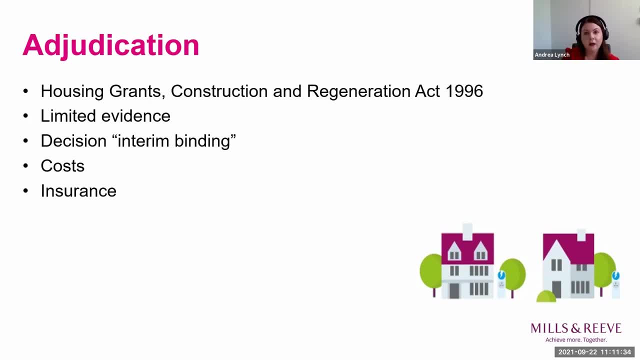 This seems like an incredibly short timescale. So I'm wondering: is adjudication, Is it even appropriate for a construction professional negligence dispute which, at the heart, stems from a breach of a professional's duties? Yeah, thanks, Andrea. 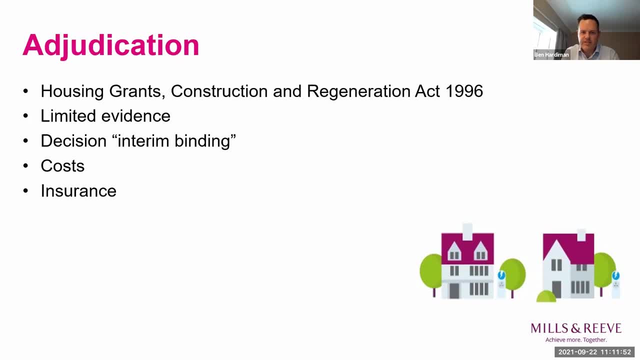 You're right, The timescale is incredibly short. The answer is start to finish, absent any agreement to the contrary within 28 days, And I think on my question with some legitimacy, how an adjudicator can properly assess the sorts of things which are necessary to resolve. 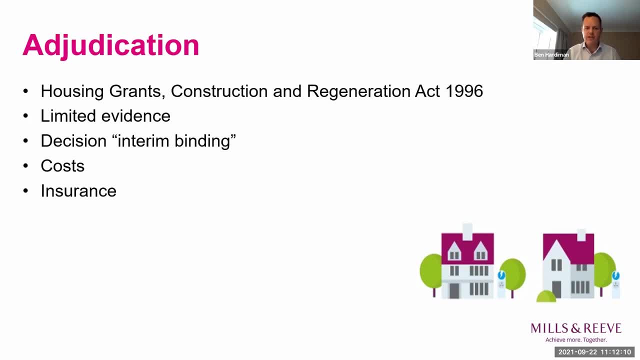 many professional negligence disputes in a construction sphere. More often than not, adjudication is used to address questions of delay, disruption, payment disputes within the scope of an ongoing project. But the reality is that this is a statutory mechanism. It was created by the Housing Grants Construction Regeneration Act back in 1996.. 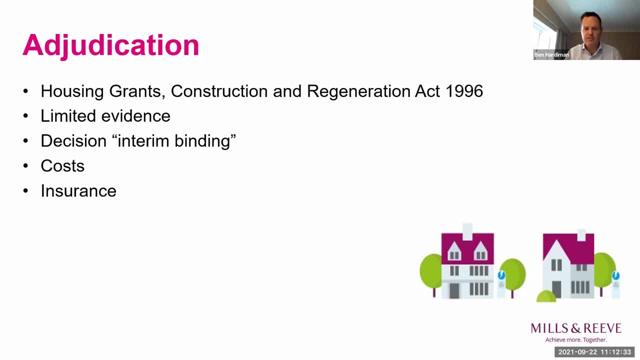 And it gives the party a right to refer a dispute arising under a construction contract. Now, the Act defines a construction Contract fairly broadly. It includes services ranging from architecture to design and surveying work, through to the building and engineering aspects of a project. 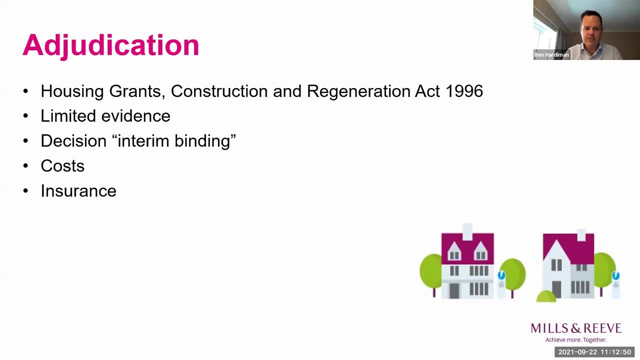 And since, subject to the usual limitation rules that Andrew referred back to, a claimant can serve, or a referring party can serve, their notice of an intention to adjudicate at any time, and that wording has been found to mean that a dispute can be referred after. 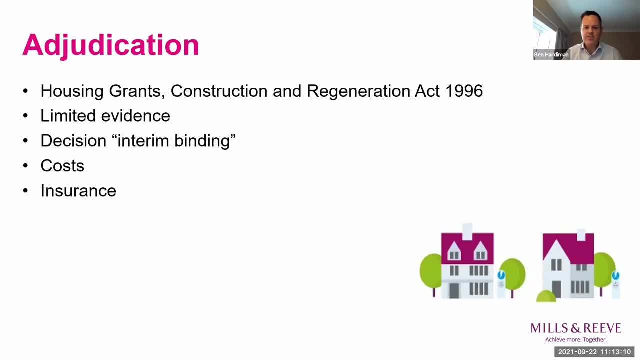 After practical completion. That's obviously relevant to PI disputes, given that many will arise from latent defects which are just not apparent prior to practical completion and may not arise for several years. So there's no express prohibition on adjudication being used for PI-related disputes. 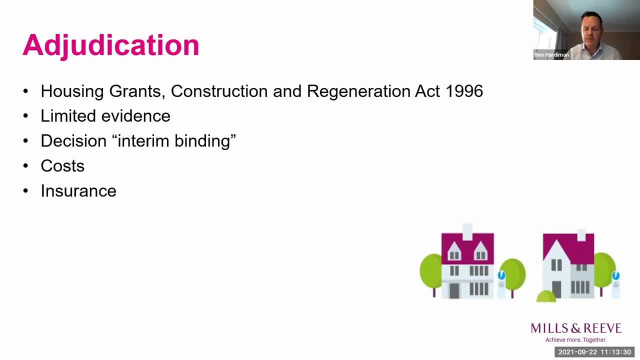 Parties can't contract out of the Act. So if there's a dispute, it is an option for the claiming party, Right? Thanks, Ben. So if you can just talk us through what the The exact procedure is for an adjudication, that would be helpful. 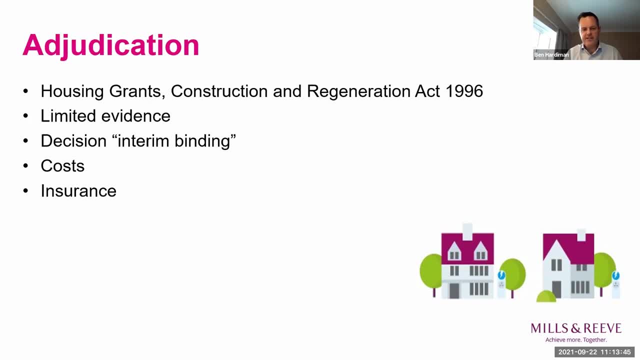 Yeah, as I said, dispute can be commenced at any time. So, bearing in mind the tight timetable which I'll talk to you about now, a referring party will usually do all that it can to ensure that its case is in order before it takes steps to commence the process. 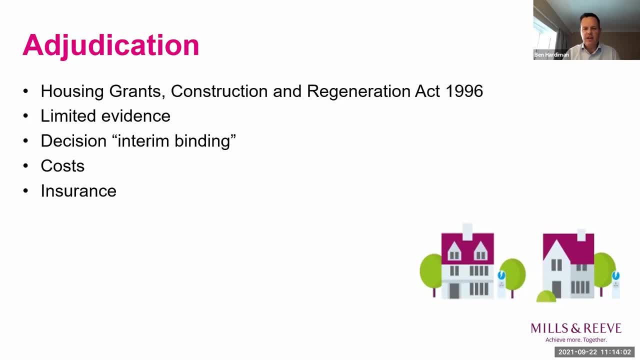 But what they have to do is to serve a notice of adjudication and they apply to a nominating body to appoint the adjudicator And that appointment must occur. It must occur within seven days. The referring party then serves a referral notice, which is the equivalent of particulars of claim, within seven days. 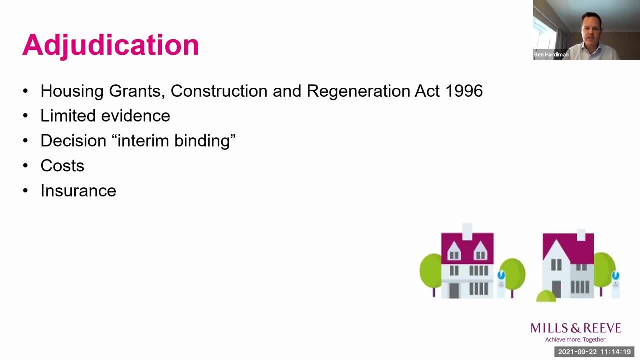 And the responding party has seven days to serve a response. So it's possible to agree to extend that, but it's ultimately at the discretion of the adjudicator to do so. The referring party will often have permission to serve a reply within three days. 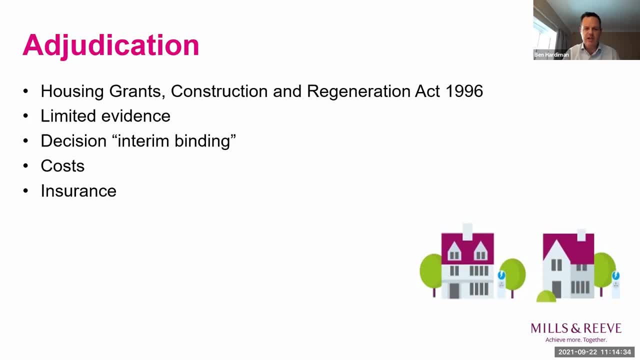 Now, these are the bits that create the issues, Unlike litigation, there's no disclosure exercise. There's no exchange of witness evidence, There's no exchange of expert evidence. Details can be submitted with the statements of case, But, bearing in mind the time scales, bearing in mind, this may come completely out of the blue. 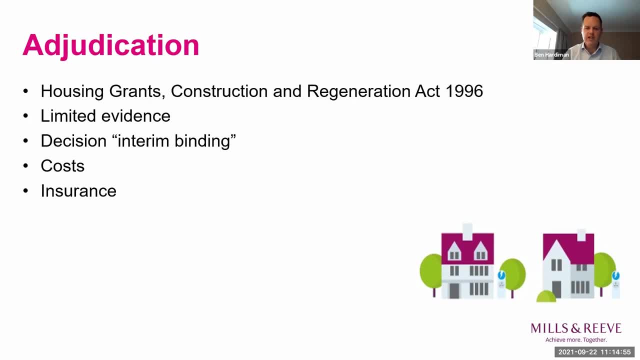 you may well really struggle to pull that together. The adjudicator can call the parties to attend the meeting, but doesn't have to, So you may well not have any oral submissions And ultimately, unless an extension is agreed by both parties, the adjudicator 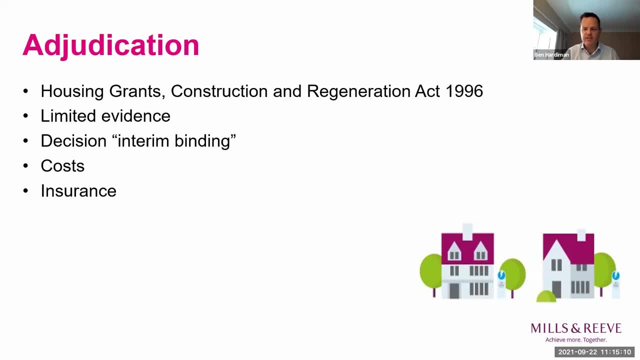 has got 28 days from service to the referral notice to reach the decision. Thanks, So clearly it's a really speedy process. So the key question is: what if you don't like the outcome? Yeah, you're almost stuck with it. 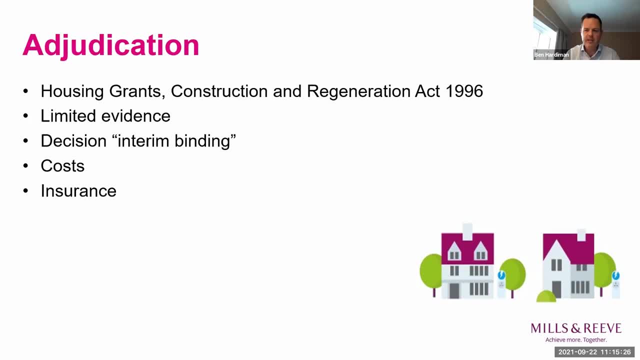 An adjudicator's award is known as interim binding. That means it's binding unless it's challenged in subsequent proceedings. So, whether via courts or arbitration, Adjudication decisions have to be enforced by the technology And construction courts. But since the court upholds the vast majority of adjudication decisions, 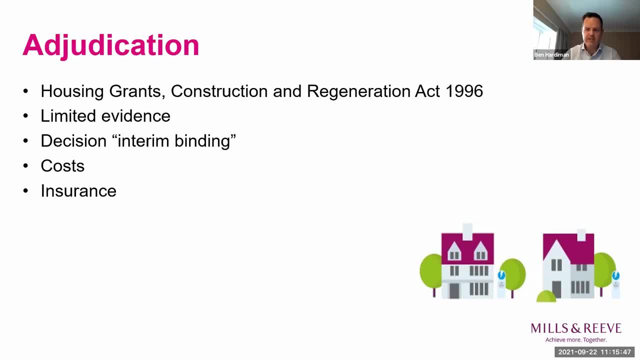 challenges are rare, And so the majority are just simply accepted. And what are the benefits of using adjudication? Ben Well, it comes back to time and cost. Ultimately, the reason adjudication was introduced back in 96 was to create a method of dispute resolution which would expeditiously and relatively 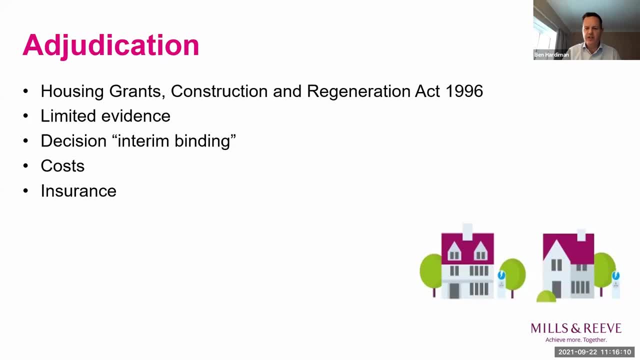 comprehensively deal with disputes. Now that's the wording of the people who prepared this. So, whilst there are undoubtedly risks for anyone entering into this process, it's often been referred to as shotgun justice because it's such a high level process because an adjudicator can't really consider the detail quite as much as a court would. 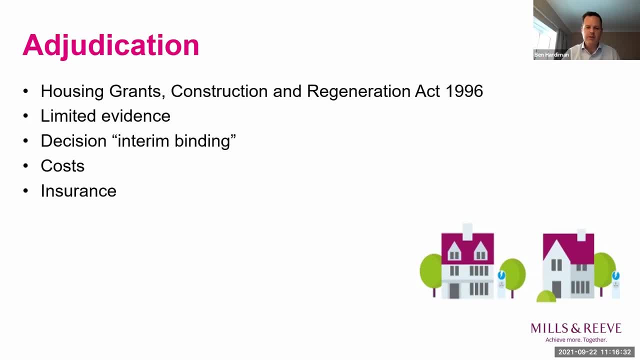 But the converse is that it is relatively quick and cheap when you compare it to legal proceedings which may take a couple of years to get from start to finish And undoubtedly very significant costs. Just on the question of costs, this is another area that can cause some tension. 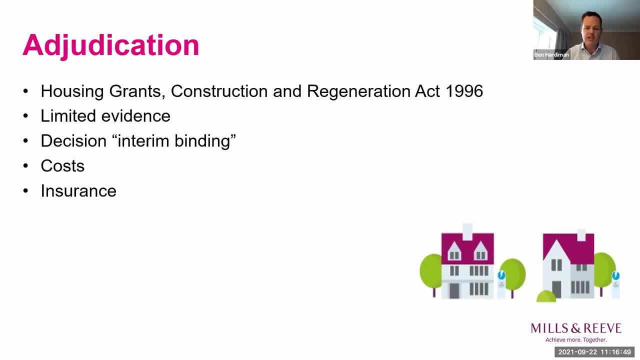 Unless agreed otherwise in writing. as part of the adjudication process, costs don't follow the event as they do in normally do in litigation, So a successful party doesn't recover their costs. Where an award might be made is that the parties are jointly and severally liable for the adjudication. 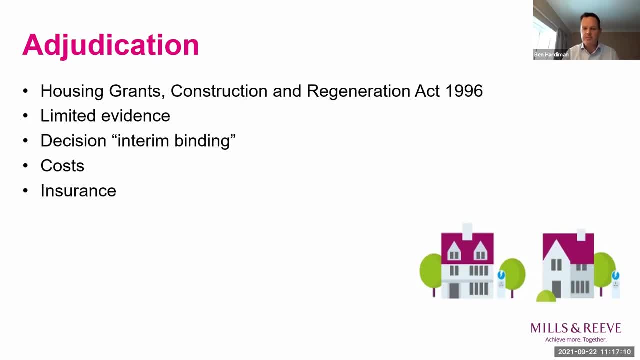 So it's not just the adjudicator's reasonable costs and expenses, but the adjudicator may well apportion the amount between the parties as he or she decides. Great, and so, just before we move on from adjudications: warning, I think it would probably be helpful for our attendees. 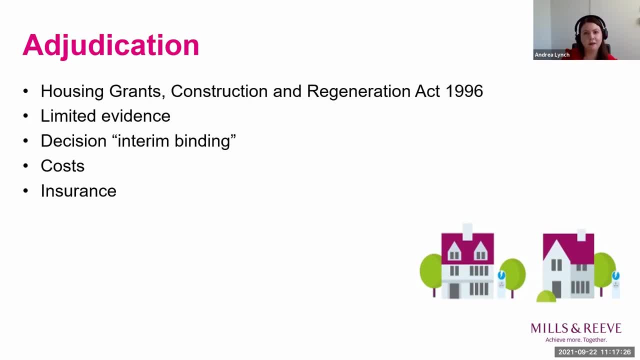 particularly in light of such tight time scales. Do you have any practical advice you would give? Yeah, it goes back to time being of the essence. read your policy, The policy of insurance. you pay for it. PI policy most normally include a specific notification provision for adjudication. so 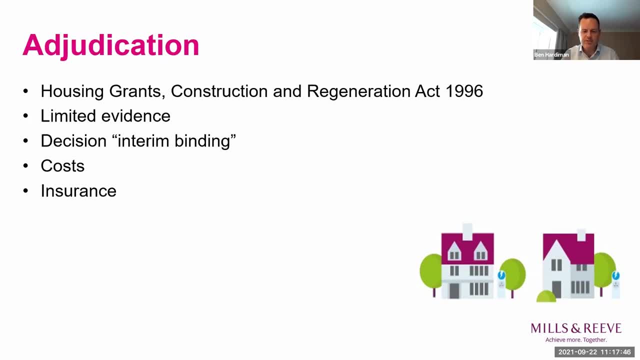 that's separate to the normal notification provisions. the majority require notification within two or three working days and that is obviously very tight. but if you don't get things moving quickly you're not going to be able to respond in time. so that's relevant both for professionals and contractors and the like on the call. it's also relevant for brokers who receive 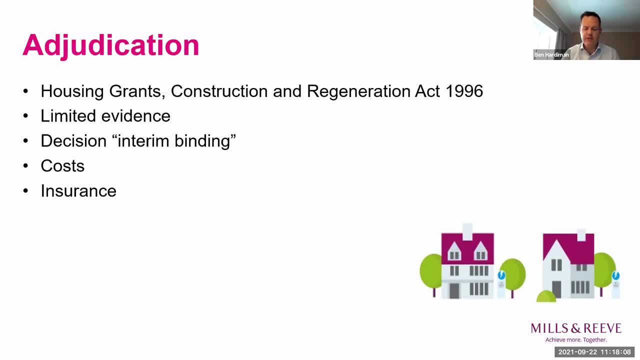 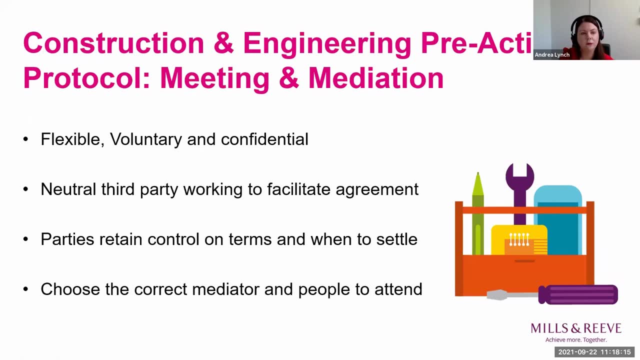 these notifications. you really need to get them over to insurers very quickly. great thanks for that, ben. that was really helpful, um andrew. we're now going to turn to the final method of dispute resolution that we're going to look at today, which is um the universally popular uh mediation. 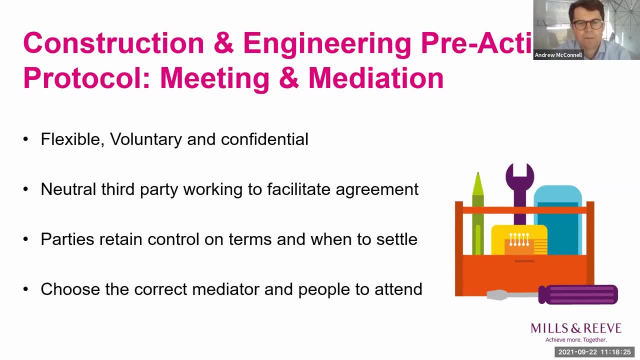 yeah, thanks, andrea. so i know uh many people will be more than familiar with mediation, but i just wanted to recap on some of the basics, essentially so, mediation is obviously a flexible, voluntary and confidential form of mediation, and it's a very important form of mediation and it's a very 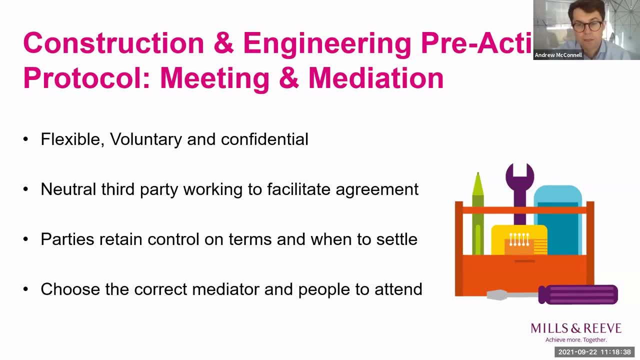 important form of adr and it involves a neutral third party being the mediator assisting the parties towards a negotiated settlement and, crucially, for a mediation, the parties retain control over a- whether or not settle and b- if so, on what terms they want to settle. and, unlike a, 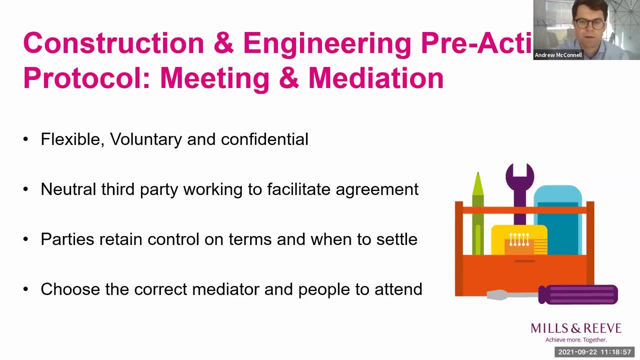 judge or arbitrator. the mediator will not decide the case on its merits, but will work to facilitate an agreement between the parties, and usually the parties to a mediation are required to treat all discussions and documents as entirely confidential and without prejudice. and what are the common purposes of using a mediation? um, i think there's quite a few, but, um, and it's probably a mixture of: 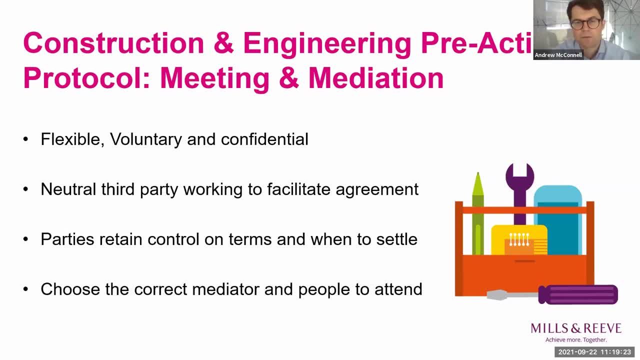 the following really: but there's narrowing the issues in dispute, which is obviously important. avoiding costly litigation and then resolving the dispute itself is, if possible. that's. that's obviously the ultimate goal, um, and it's important to note, and perhaps it's it's why mediation is so. 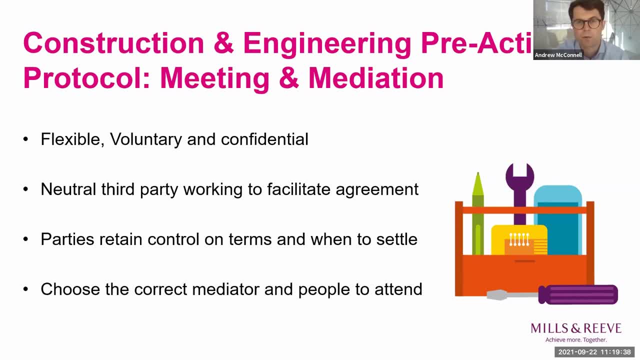 popular? it's because it's suitable for all kinds of disputes, whether it be small claims of a low value or, you know, high value, quite complex and technical construction disputes. and what would you say are the the main benefits of of using mediation, comparing it to the other forms of? 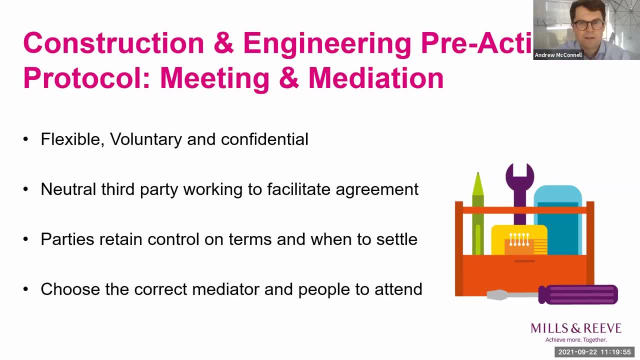 dispute resolution that could be used well, i think there are plenty, so, um, business relationships can be preserved- that's obviously important given my confidentiality point from earlier- and the parties have also got complete choice over the selection of a mediator. um, obviously isn't the case when it comes to a trial judge, as much as we'd like it to. 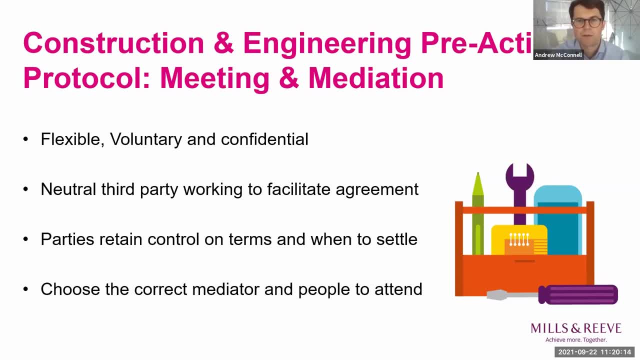 be. so you can pick um an arbitrator with a suitable approach and suitable expertise. sorry, a mediator. i'm getting confused now, but obviously um often mediation avoids um expensive litigation, although there are obviously legal costs um associated with preparing for a mediation, and you've got those of the mediator themselves. uh, mediation can. mediation can provide a speedier 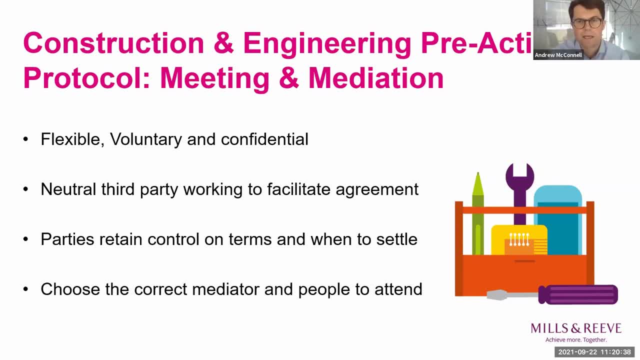 so we're talking a number of weeks to to really um get a mediation um sort of arranged, which obviously isn't the case with court proceedings can take much longer. a mediation has a high success rate and i think, quite importantly, even if a mediation doesn't resolve the dispute and 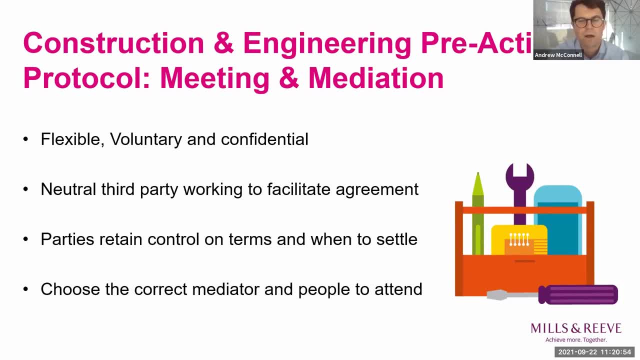 you don't end up with a settlement. it's often quite a helpful process for the parties just to get together, listen to each other's positions and perspectives. that can, that in itself can can form a very beneficial process for everyone involved. yeah, great thanks, andre. um, i think we've got another quick poll, um, which should hopefully be on your screen. 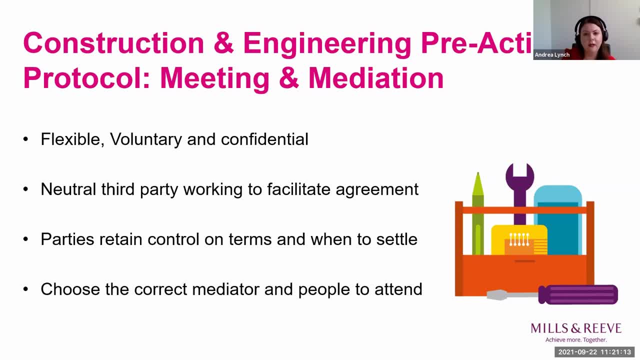 now. um. so for those of you who've attended mediations, um, the question we've got is: which of the below factors would you consider most essential to productivity of a mediation, so the right mediator for the case, preparation of parties and management of settlement expectations? um a sensible starting point in terms of opening offers, the fact that it's binding. 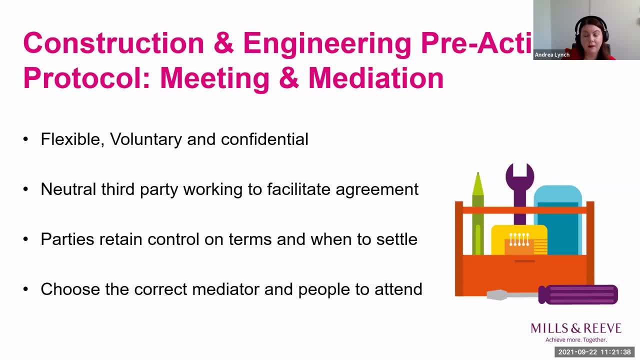 a strong mediation position statement and one that's exchanged in advance. a large number of people are voting here- quite a mixed bag, which is um a lot of. you think the choice of mediator is a priority preparation as well. um, andrew, um 20 percent of our attendees. 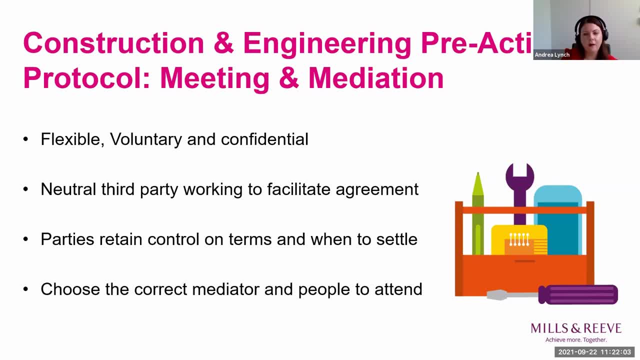 this morning are suggesting that, uh, one of the factors that's most essential to productivity of a mediation is the fact that mediation is binding. do you want to talk to us a bit about that? yeah, i mean, we threw that in as a bit of a red herring because, uh, mediation is obviously not. 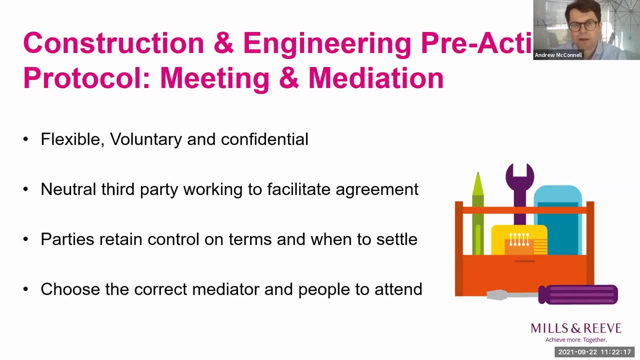 uh, not binding, as i mentioned earlier. so that's something to bear in mind when going along to a mediation, that there's no obligation on the parties to come out of it with a settlement. and i think it's quite interesting as well- the poll revealed that. you know, choice of mediator is an important 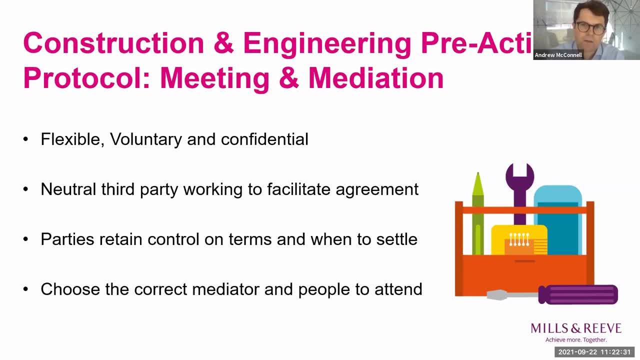 factor and i think, i think that's true and i think you know panel solicitors- we'd always have a selection of recommended mediators for a particular party, and i think that's a very important factor in the dispute. yeah, definitely, definitely, um, just finally then um, andrew, again, a key question is: do 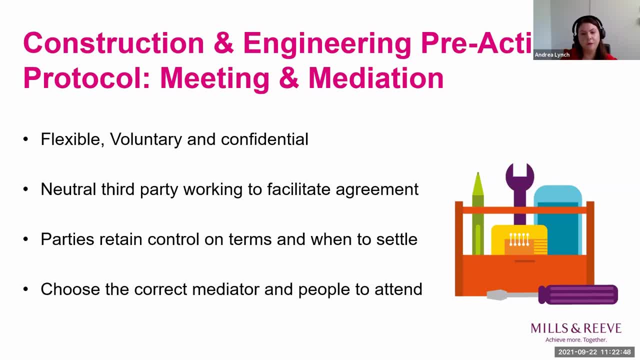 you have any from your experience? you have any practical tips, um, in terms of preparation and attending a mediation that makes it more successful? yeah, um, you know, as we've alluded to the right mediation for the right case- sorry, the right mediator for the right case- so, um, someone. 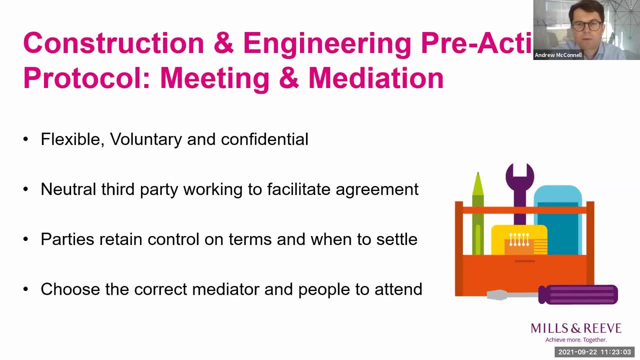 who might be a straight talker, could be sensible and appropriate for a particular case. on the flip side, you might need, um, somebody who does a bit more hand-holding, for example if a claimant or other party isn't legally represented. so this obviously depends on the facts of the case. 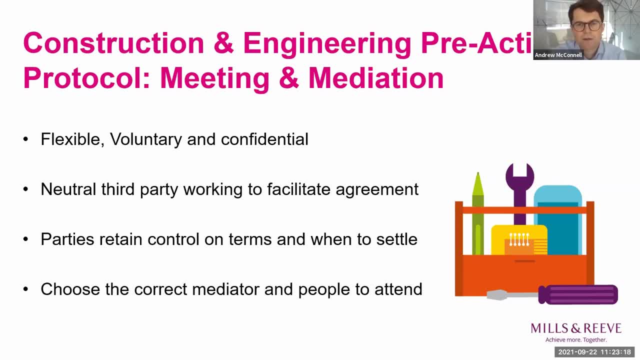 uh, you obviously need to think about who's going to attend. so are you going to have lawyers in attendance? that's quite common, of course- um directors and officers of your clients, claims handlers for insurers, who can be very important on the day in terms of negotiations and settlement. 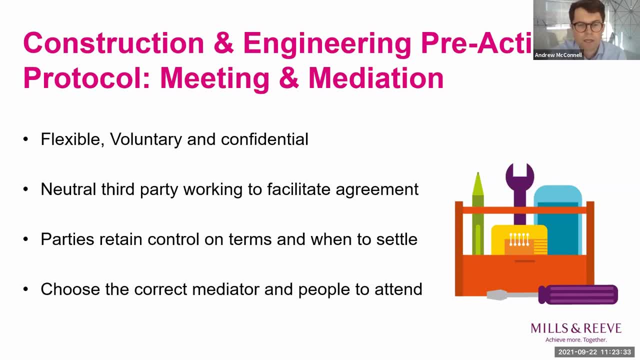 authority and insurance brokers to help the insured through the process. um, another factor is that there's a lot of people who are not going to be able to attend a mediation for the right case, so you need to think about who's going to be able to attend a mediation for the right case. 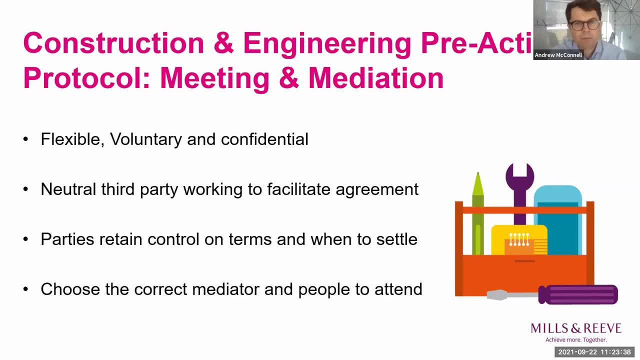 another factor is whether it will be online or in person. i think we'll probably see a bit more of a return to to sort of in-person mediations after the pandemic, but in recent months we've obviously gained quite a lot of experience in conducting mediations via zoom and they have proved quite 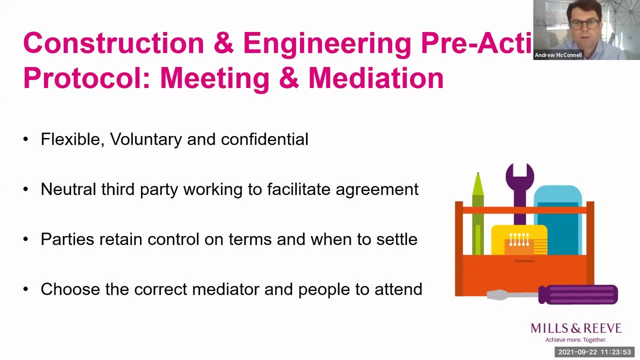 effective as time has gone by, and the mediator can obviously utilize breakout rooms to maintain confidentiality and things like that, so they can be quite appropriate for the right case if you do them virtually. another thing to consider is whether there'll be opening statements in a sort of preliminary session. they can provide a really good opportunity to get things out in the 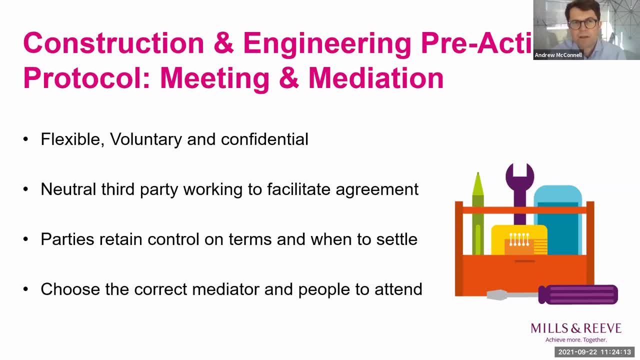 open and confirm that the parties are attending in good faith. but you don't want to use them as an opportunity to just antagonize each other and, you know, rehearse previous arguments that you've already exchanged in correspondence. so it's something to think about. another factor is 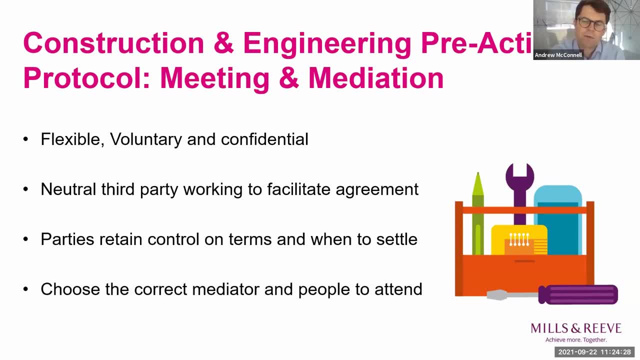 settlement authority. do you have the requisite settlement authority before the mediation, and by that i mean from any insurer clients and indeed from the insured client. but also, do you have somebody there authorized to sign the settlement agreement once it's finalized? that can be an important factor on the day. and just a final tip is is sort of having a hard copy draft. 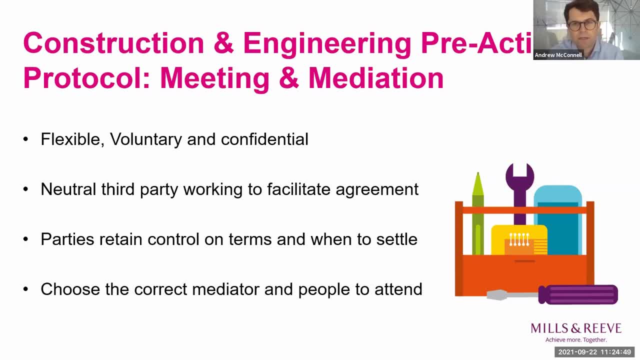 settlement agreement ready to go on the day, because there's nothing more frustrating than reaching a settlement but then having to spend quite a few stressful hours at the end of a long day scrambling around trying to get a settlement agreement together. so that's something to be avoided, with a bit of preparation, i suppose. yeah, definitely, andrew, definitely. um, thanks, andrew, and. 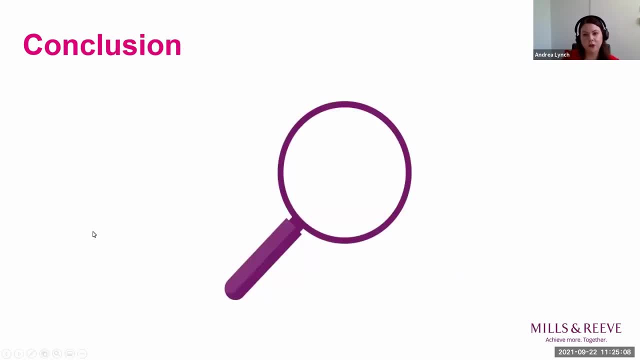 thanks also to ben um. into today's session we've not touched on the other main method of dispute resolution, which is of course court proceedings. we will cover those in in later breaking ground sessions. but it's important to note that the main reason that these alternative forms of dispute 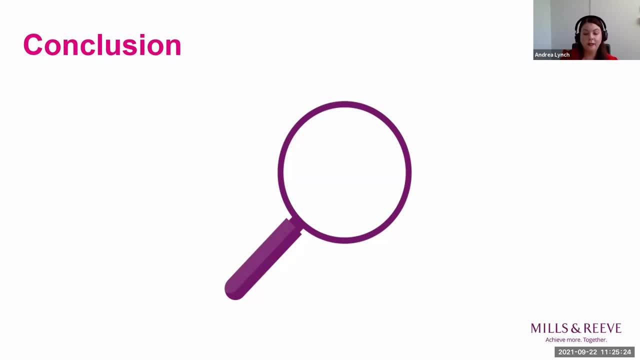 resolution that have actually been created is to try and avoid the lengthy um and expensive court proceedings. um costs and speed are a key driver in these alternative methods of dispute resolutions, but parties should be able to do so, and i think that's something that we need to. 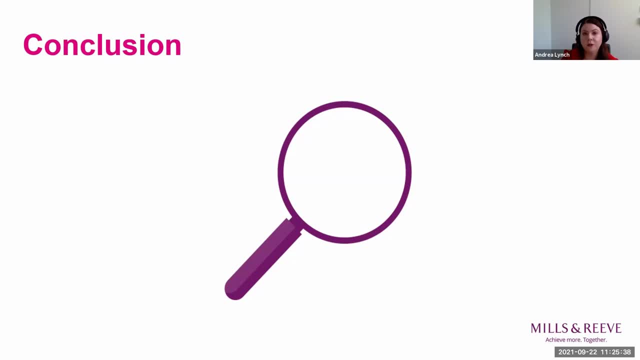 look at as well, and i think that's something that we should be careful to seek to match the resolution process to the dispute itself and also ensure that any contracts that you're entering um in in a construction setting do contain appropriate dispute resolution clauses. picking the right process may be key to the success of the of achieving resolution off a. 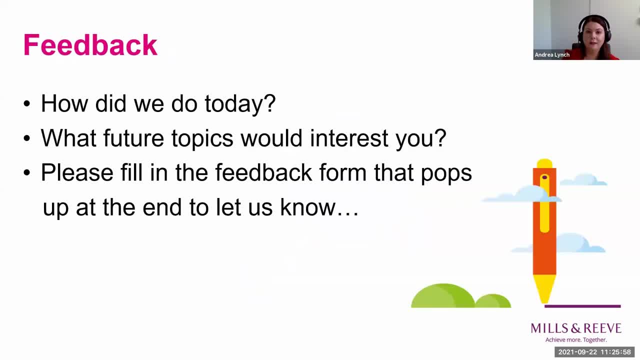 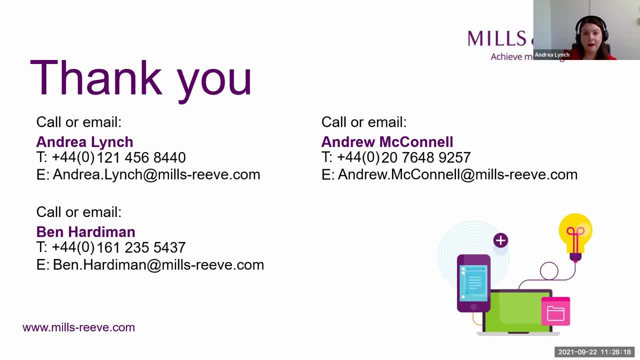 dispute. um, that's all we've got time for today and thank you so much for joining us this morning. the next breaking ground webinar series will explore the light and the dark side of dispute resolution and the life cycle of a claim, of a typical professional negligence claim in a construction. 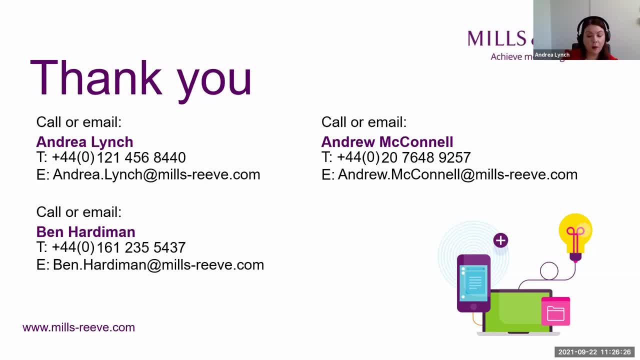 setting from notification through to settlement. the first webinar of the new series is titled first steps when notice of a claim lands on your desk, and that's going to be held at 11 am on the 13th of october. we do hope you can join us then and wish you a good rest of the day.